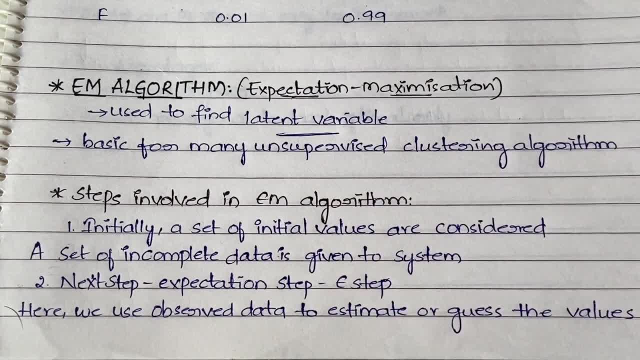 And it was also basic for many unsupervised clustering algorithms. So you have so many unsupervised clustering algorithms, right? So for all those algorithms, this EM, EM algorithm, you know what unsupervised are in machine learning, you have three types: you have supervised, you have unsupervised, you have reinforcement. 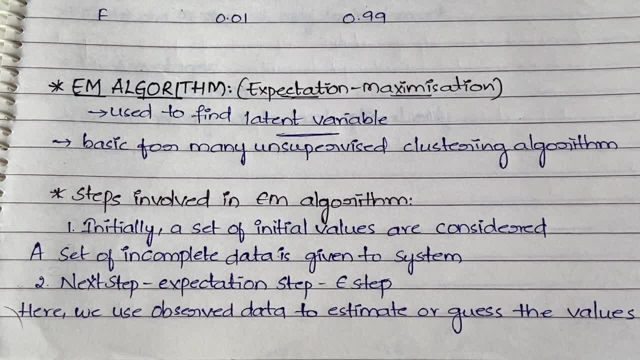 So in that it is a basic, it is a basic concept for many unsupervised clustering algorithms. Okay, and now I'll tell you what latent variable is actually. So latent variables are nothing, but you cannot directly observe that here. you cannot directly derive those variables. 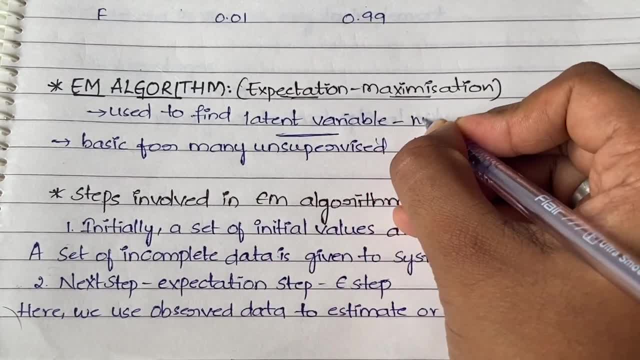 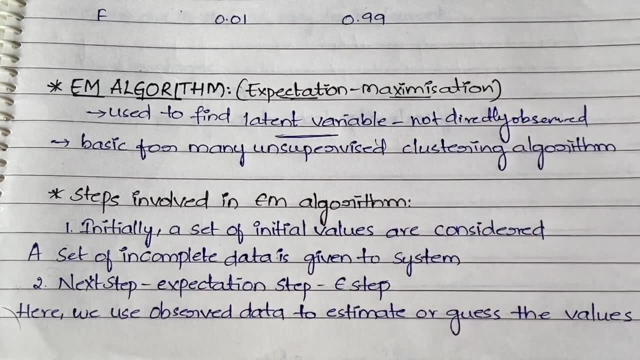 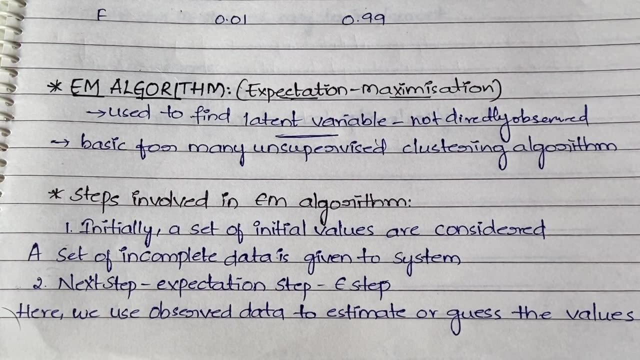 Okay, so these latent variables are not directly observed, Then how do you get them? How do you observe them? How do you get these, get their values? You can infer them from the other observed variables, that is, the previously observed variables which you have in your system. 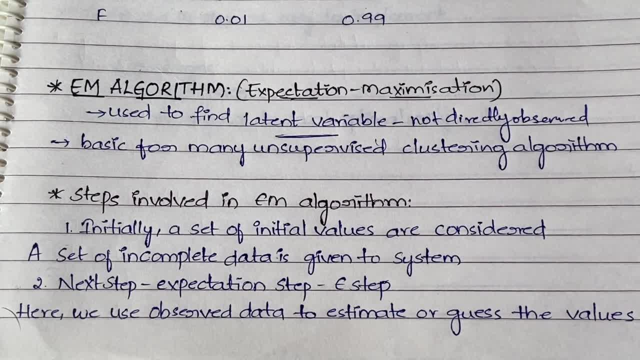 You can infer the value from those variables. Okay, so this is how EM algorithm works on. It is used to find out the latent variable. and what do you mean by latent variable? The variables which you cannot directly infer. you need to depend on some other variables in order to get the value. 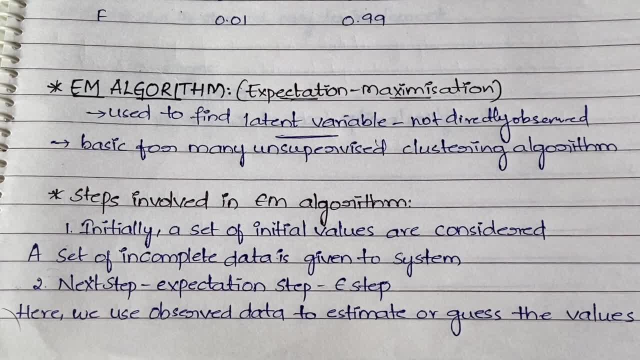 In order to observe that value. Okay, done. So this is about the EM algorithm, and in this video, you will learn about what are the steps involved in EM algorithm, What is the usage of EM algorithm, What are the advantages and what are the disadvantages. Okay, so these all you'll be learning in this video. 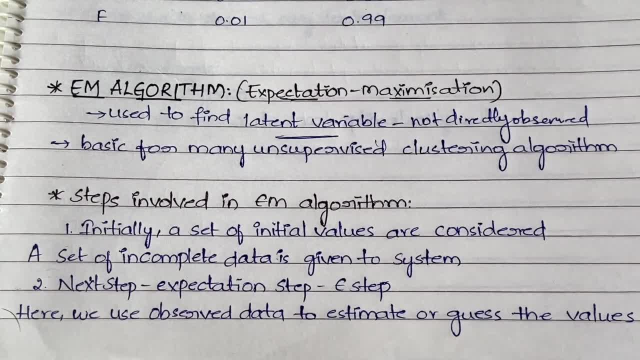 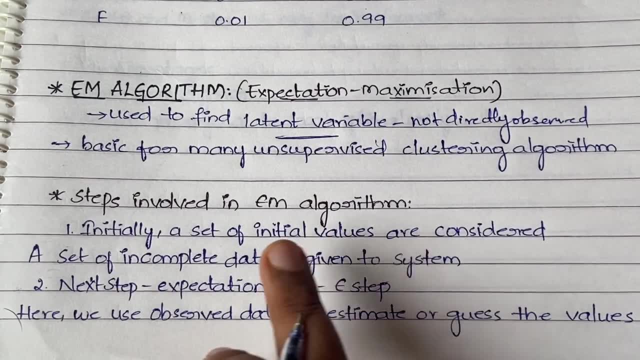 So first let us see what are the steps. We have actually four steps, very simple steps. You can easily understand them. First, what you have to do is initially a set of initial values are considered. So first you need to consider a set of values. 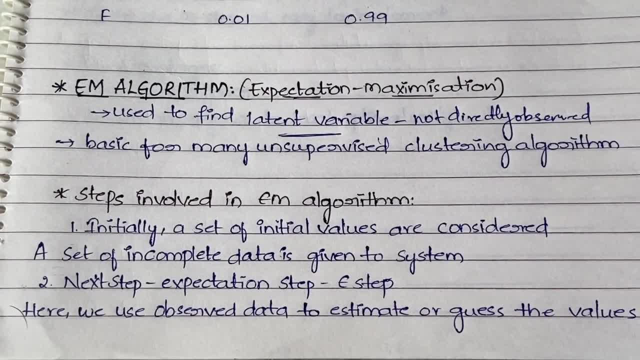 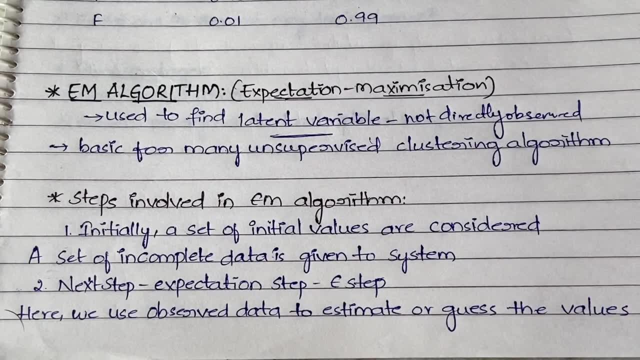 you need to consider some incomplete value, some initial values, and you need to give that to the system and all those values are actually incomplete. okay, so next, in the second step, what you will do is: second step is the expectation. so here means expectation maximization, right, so the second step. 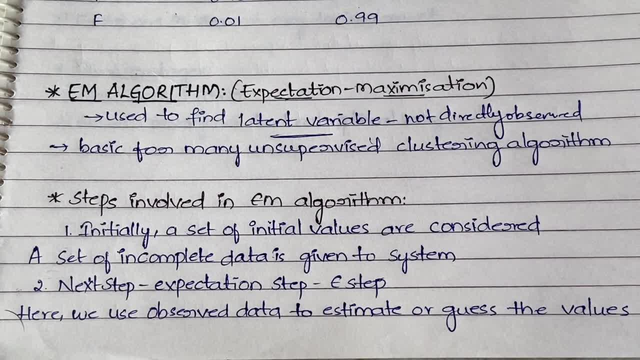 is expectation. so in expectation step, or this is also called as e step. so in this step, what you will do is you will be using already observed data to estimate or to guess the values of the missing or incomplete data. so here we have incomplete data, right? so in order to guess the value of this, 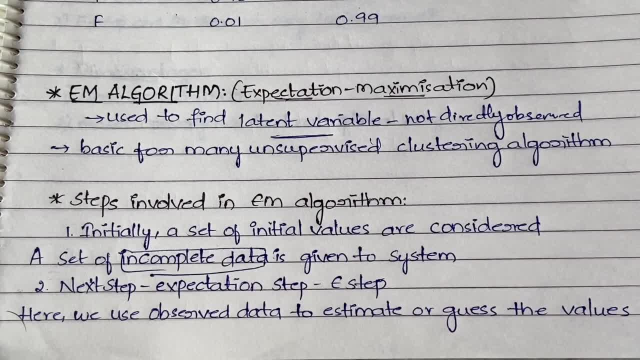 incomplete data. okay, you in, uh, you know, in order to give the values to that incomplete data, you will be estimating or you will be guessing the values based on the previously observed data. so, with a reference from the previous data, with the, you'll be using that data and you'll be guessing. 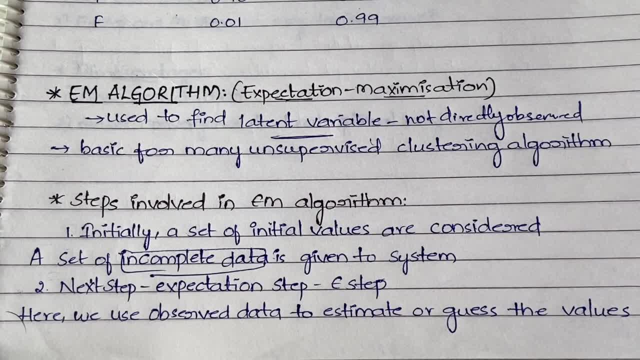 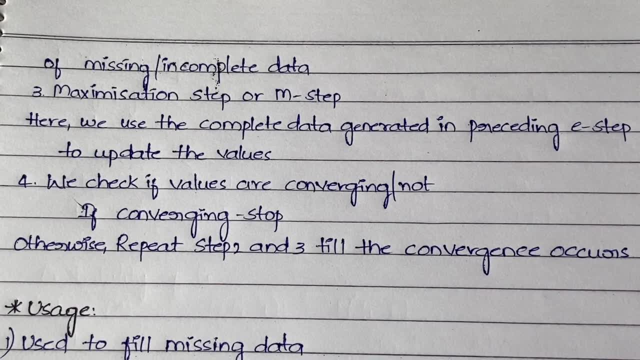 the values or you'll be estimating the values for in the incomplete places done that is the expectation step or the e step. in the third step, that is nothing but the maximization step, which is also called as m step. here, what you will do is: here we use the 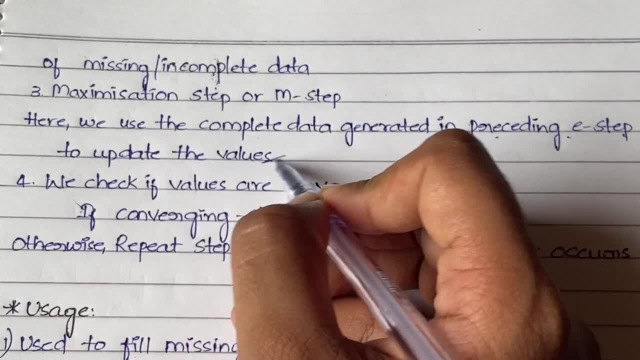 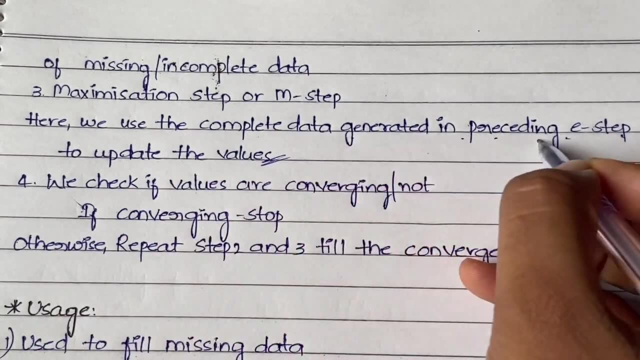 complete data generated in preceding e step to update the value. so, whatever the values are there, so you will be updating all those values- see the complete data generated in the preceding e step- and update the value. some of the values are missing right, so some inconsistencies will be there, some. 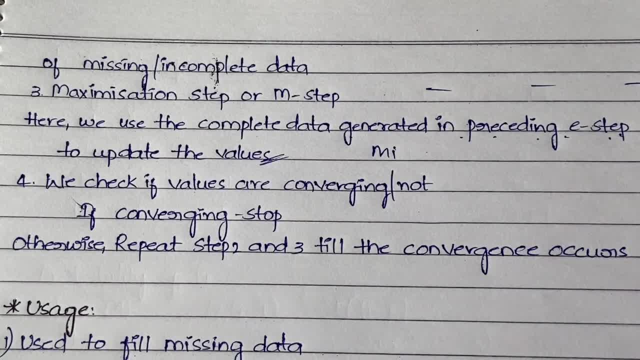 missing data will be there, so you will be updating all the data. so, based on the previous data, we have filled up the missing positions in the previous step. here. what you will do, you will be updating. okay, so, and so was. previously it was missing. now it got some value, so like that you will be doing. 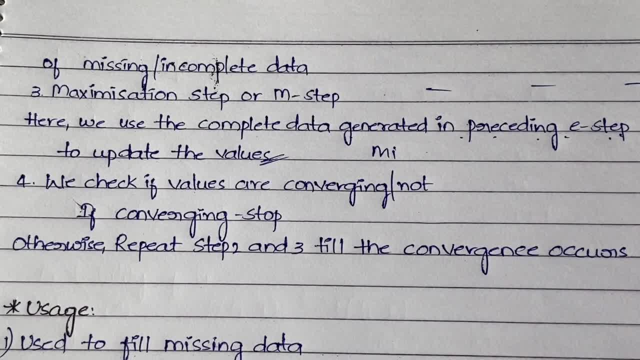 all the updates in the maximization step, okay. and in the fourth step, what you do is you will be checking if the values are converging or not. right, if you find the values are converging, then you can stop the process. if you does. if you don't find that the values are converging, then you need. 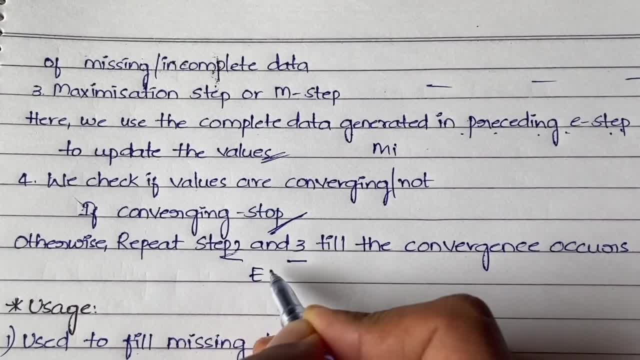 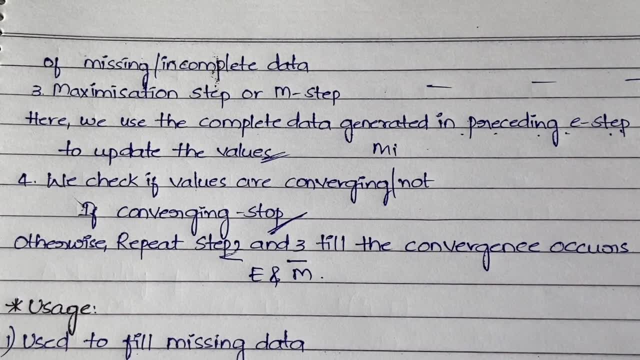 to repeat the step two and step three again, that is, you need to repeat expectation and maximization again and again, until and unless the values are converging. okay, expectation, expectation in the sense, what you have to do, you need to fill up the missing data and in maximization, you need 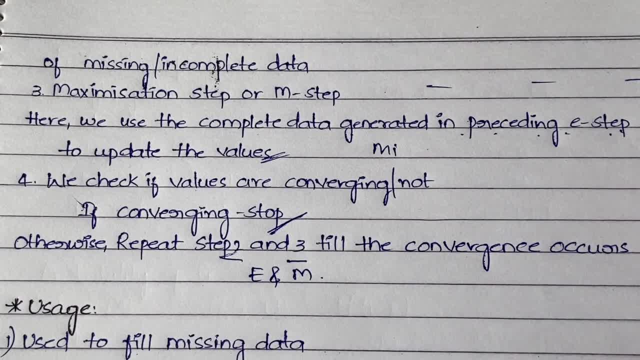 to update the data. complete data you need to update right. so any effect, if there are any changes, all those changes are to be updated. and once you do the updation task you have to check for the convergence among the data. if there is no con, if the sorry, the values are converging, then 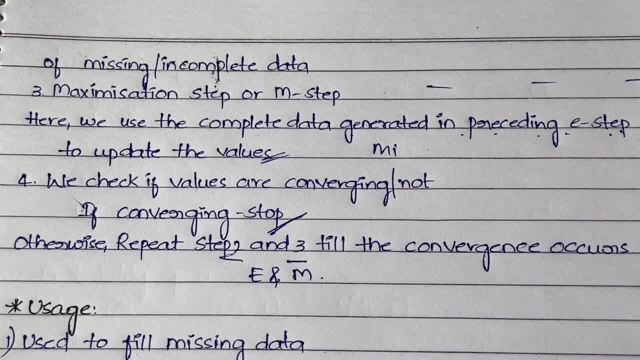 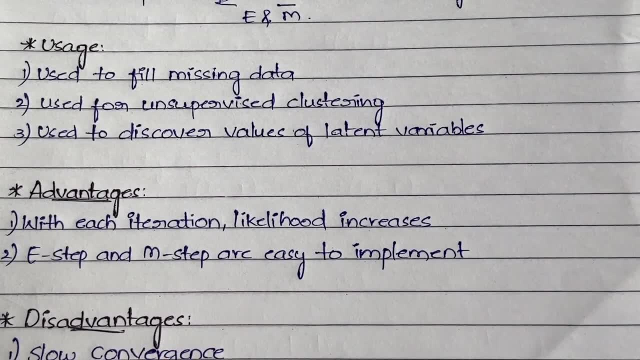 you can stop. if the values are not converging, then you need to repeat and repeat the process again and until and you you find the convergence okay. the next comes the usage. so what is the usage of this? um, you know, em algorithm, expectation maximization algorithm. so it is used to fill the missing data. 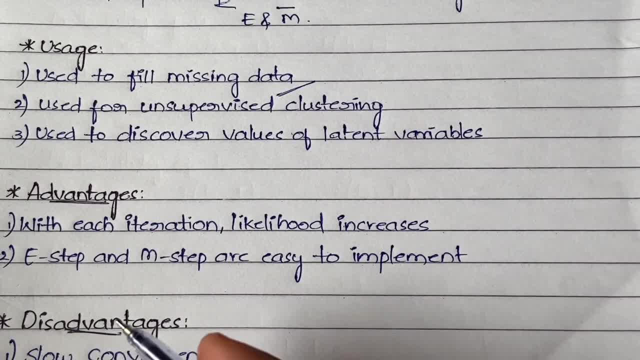 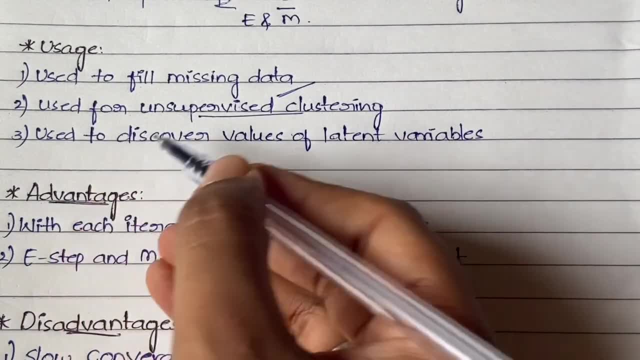 that is what we understood now in the expectation step. that is what we do right. and it is also used for unsupervised clustering. that is what i said in the beginning of the video and the again this one also you can you know this. it is used to discover the value of the latent variable. this: 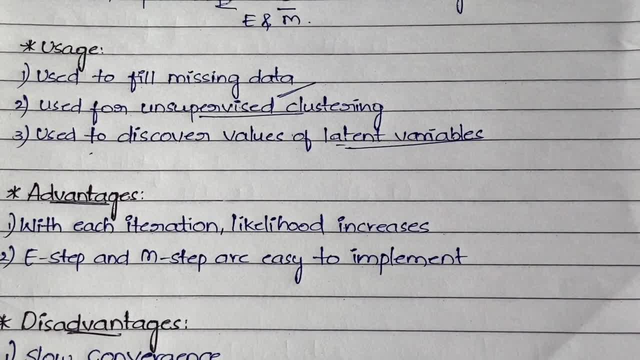 also i said at the beginning of the variable. so what do you mean by latent variables? the values which you cannot directly observe. you need to depend on some other values to get the value of this variable. then that is called as a latent variable, so you can discover the values of the. 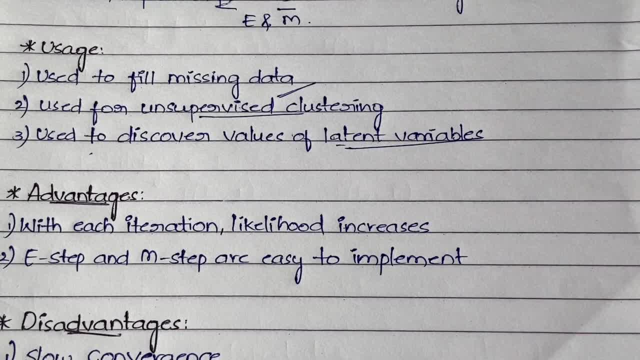 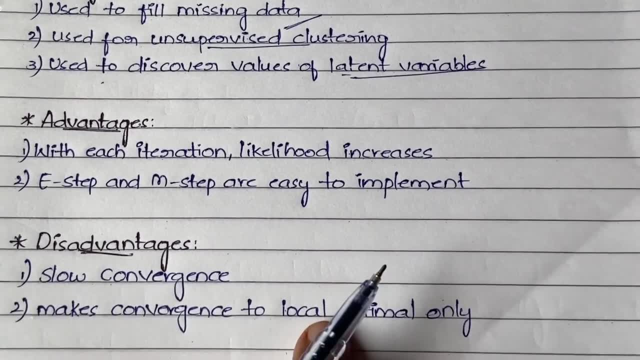 latent variables by using this em algorithm. okay now, so that these three are the main, important and common usages you have with the em algorithm done. now let us see the advantages. so with each and every iteration. so where do you find our iteration? so in the conversion step, if they are not. 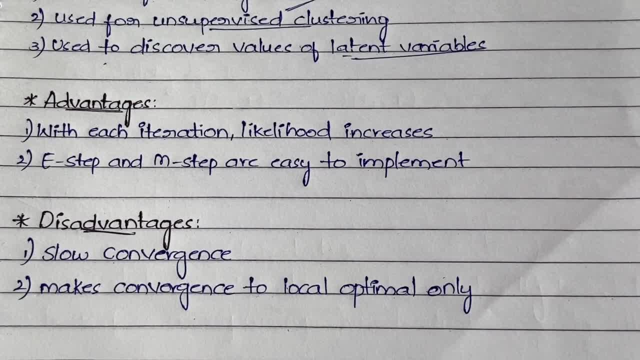 converging, you repeat step two and three, again and again, until and unless you get the convergence right. so with each and every iteration the likelihood is that you get, the value of the latent variable will increase. likelihood of the hypothesis will increase with each and every iteration you do. 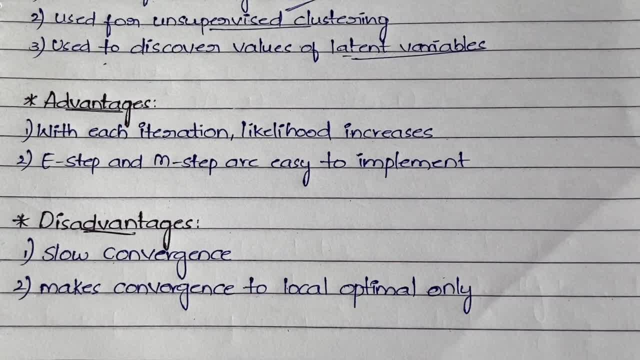 right. so for each and every iteration, the convergence keep on reducing right, and a step and m step are easy to implement right. so a step, that is the expectation step, and m step, the maximization step- you can easily implement them instead of performing so many complicated calculations. of course you need to perform some calculations as well, but still they are about easy. 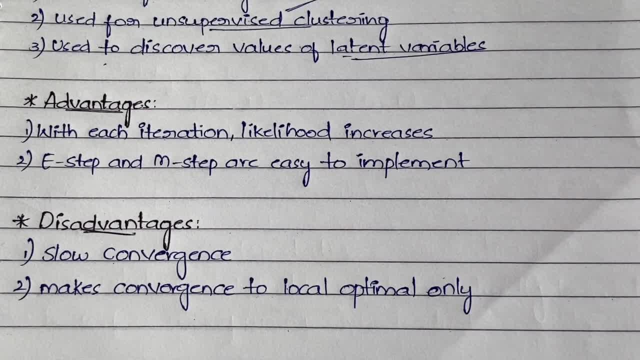 easier to implement when compared to other algorithms. okay, now coming to the disadvantages. so first thing is slow convergence. so main thing is what we have. we are checking for the convergence, but here we get the convergence very slowly. that is, you need to perform so many iterations in order. 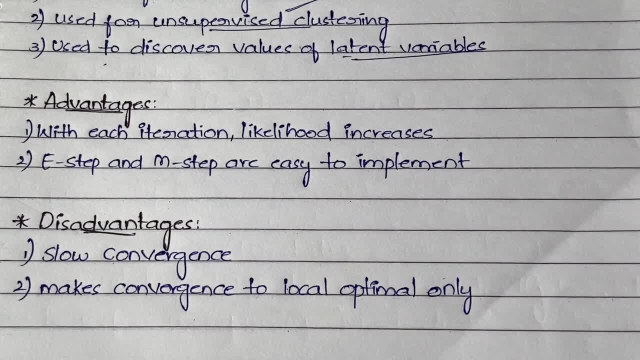 to get convergence right. and the second is it makes convergence to local optima only, that is, only to the local one, not to the global optima. okay, so the convergence which you are doing, even by number of, even though you are making so many iterations, but still you will be able to make up.